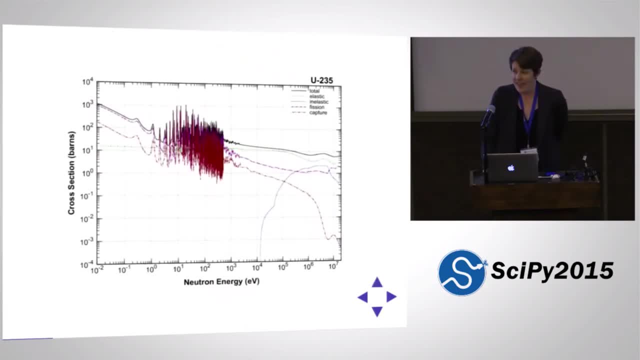 It depends on a whole bunch of variables and we call it sigma. Okay, and that cross-section embeds a whole ton of physics. So you have elastic parts of that cross-section, inelastic parts of that cross-section. So those of you who are physicists are like: 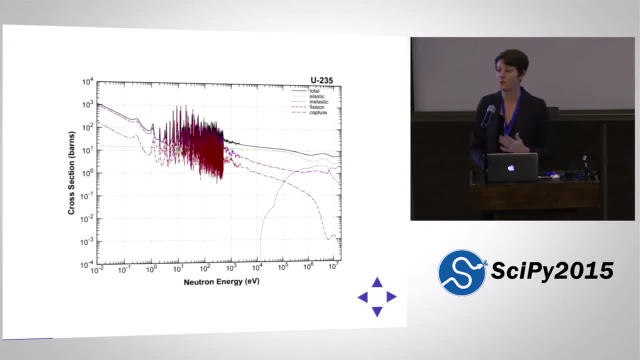 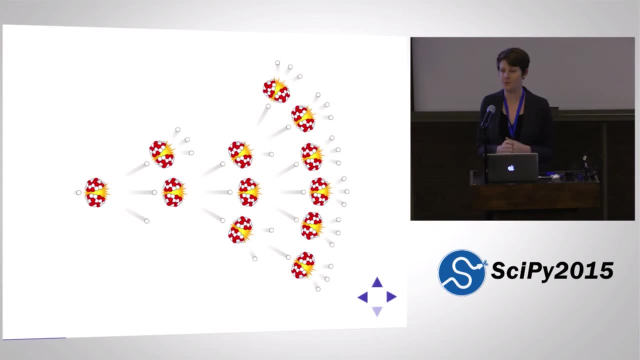 okay. so cross-sections are the probabilistic black box of nuclear particle interactions, And more than one fission will happen after those secondary neutrons are spit out. So once the fission occurs, you have the first neutrons that come off of the initial fission. 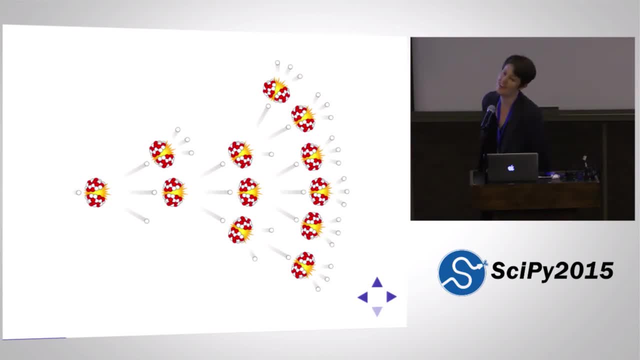 Those neutrons themselves can generate more fissions And that's how you get the nuclear chain reaction. So in a reactor, electricity is made when the heat from this nuclear chain reaction warms up some water somewhere in the system, spins a turbine and puts it into the lights. 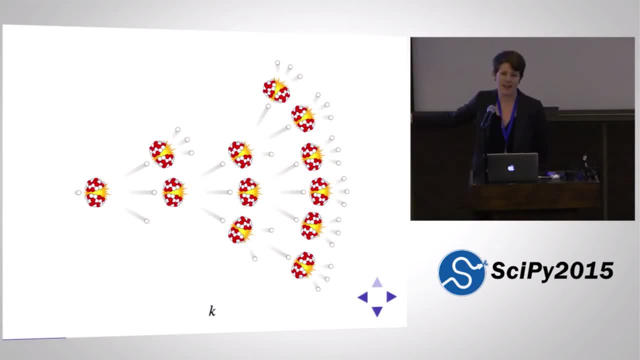 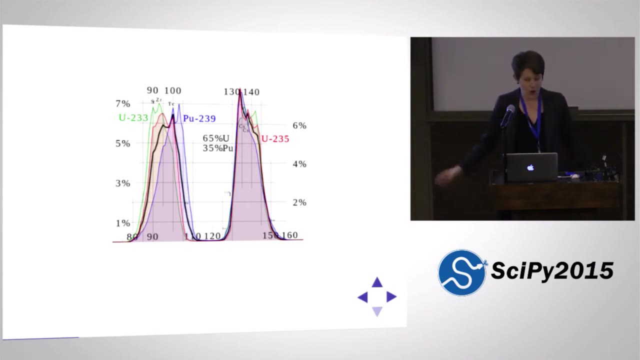 So we call this nuclear chain reaction stability k. Okay, so this is a variable that you're just going to have to keep track of a little bit, and when it's one, the reactor is critical. So at the end of this chain reaction, a whole bunch of isotopes are produced. 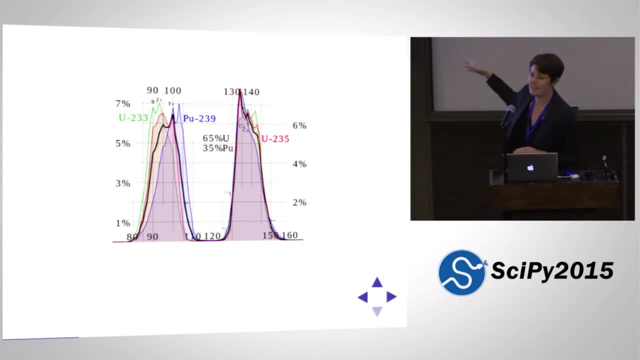 So this graph is on the bottom axis the isotopic number there, and on the y-axis you have the percent of the isotopes that are produced, And it's an interesting shape. It's not consistent. The halves are often one-third and two-thirds sized. 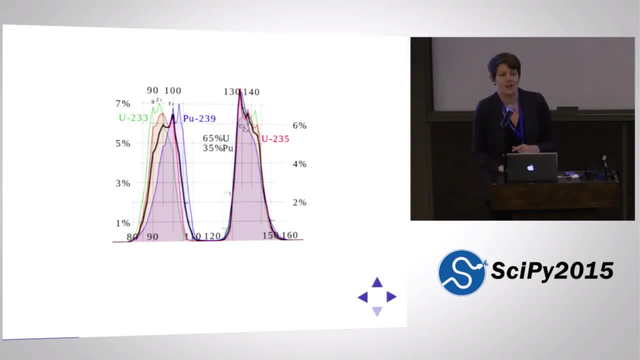 Anyway, all of the isotopes in the periodic table are made in a nuclear chain reaction And we're going to call the isotopes I. So one other interesting fact is that once that isotope has been made out of the fission, so that piece of the isotope 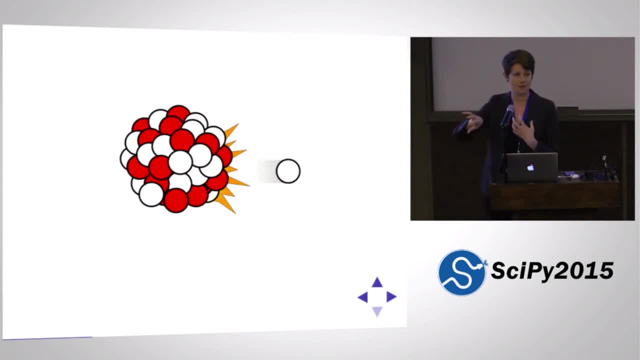 one of the two pieces that broke apart in the original fission. once that's been made, sometimes it's also unstable and it kicks off what's called a delayed neutron. So there's the initial neutrons that come off of the fission. 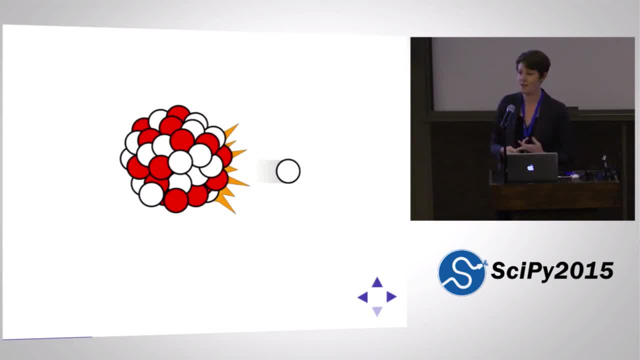 and sometimes the secondary isotopes that are made in that fission are unstable enough to kick off a third sort of a tertiary neutron, called a delayed neutron, sometime later. And so this is an interesting kinetics problem. You might call this dynamics, but the time process of this is quite interesting. 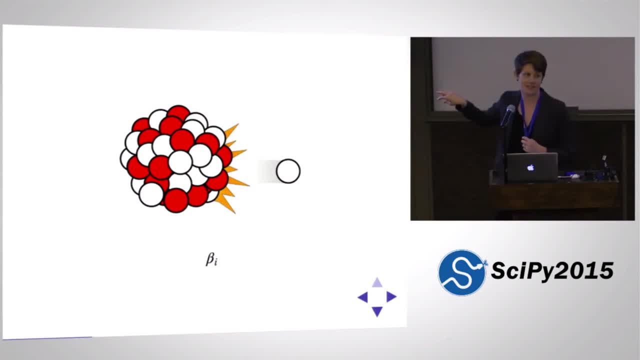 And we're going to call the probability that this neutron kicks off an isotope beta I. You don't have to keep too much track of it, But ultimately all of this stuff, the likelihood that this reactor is going to increase or decrease in power. 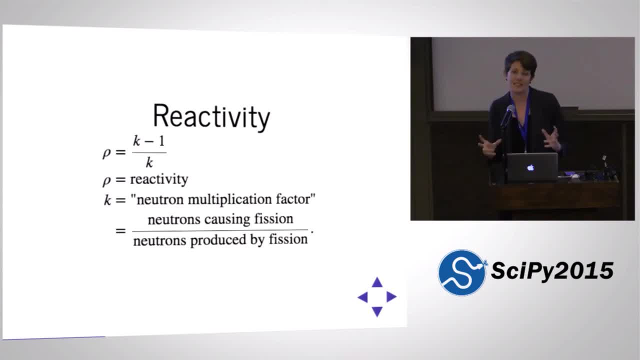 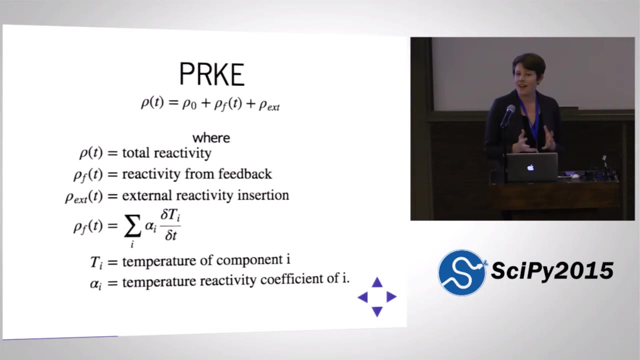 all of that contributes to something called reactivity, which is a function of k, that criticalness of the reactor, And we call k the neutron multiplication factor, and we call rho the reactivity, And now we get something complicated. So all of that combined plus some external reactivity. 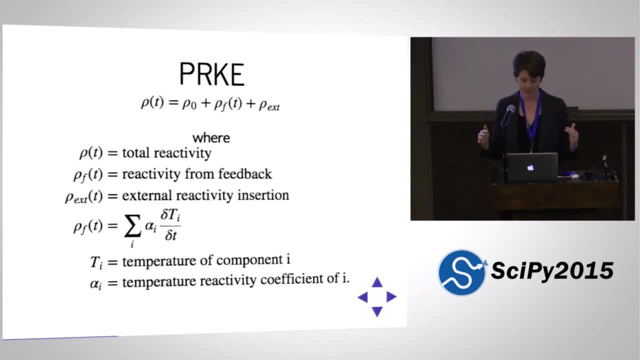 can contribute to the total power in the reaction. There's the base reactivity in a critical reactor, plus reactivity from feedback- and we're going to get into what that means- plus external reactivity which might come from dropping a control rod or lifting one out. 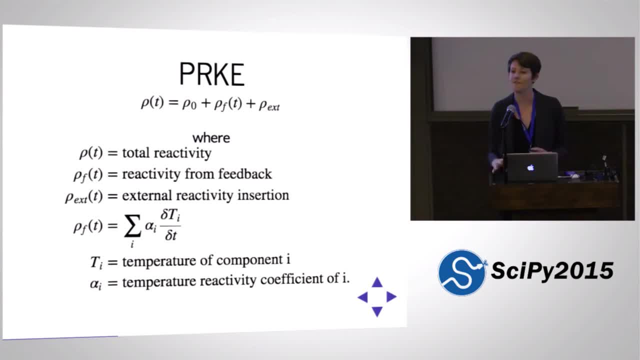 And that happens because different materials have different probabilities of fissions and different distributions of the isotopes that come out of them and everything. So keep in mind that these become the key equations in the later solution. So, anyway, it all depends on temperatures. 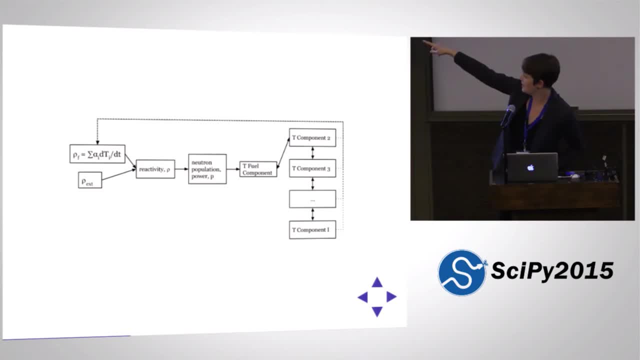 and it all feeds back. So reactivity over here feeds the neutron population, which is power. that k And each of the temperatures respond to that power, because power is heat. And so the temperatures of the various components in your reactor, like fuel or coolant, respond to the power by increasing if the power is increasing. 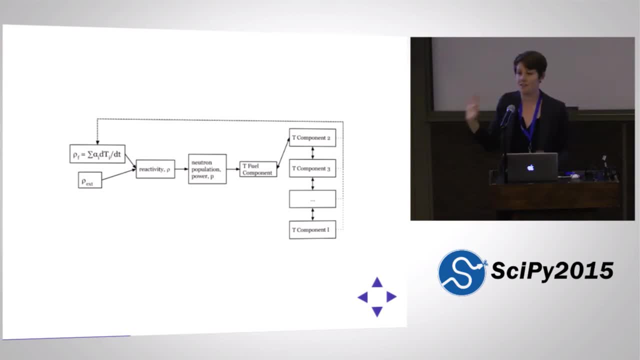 And so all those components, some of them have different reactivities, the likelihoods of kicking off more neutrons or fissioning, and that feeds back into reactivity. So this loop, this reactivity feedback, is a very interesting dynamics problem. 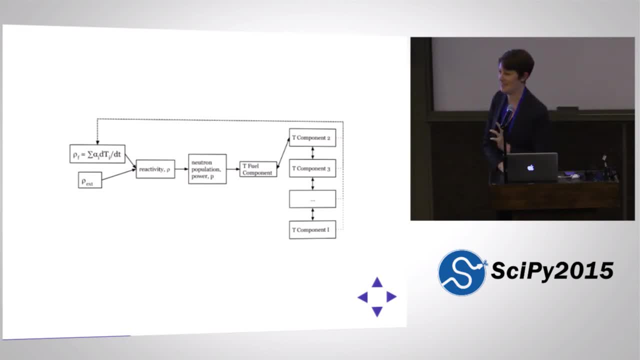 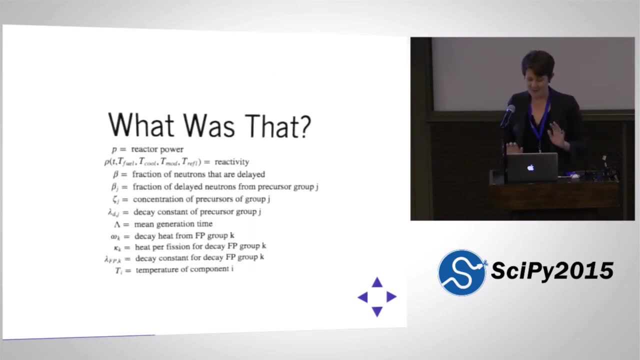 which is what PERC models. So erode a piece of Python code, of course, to model this matrix equation. We don't need to go into it right now. Just note that there's these descriptions that I've just given you about how the reactor functions. 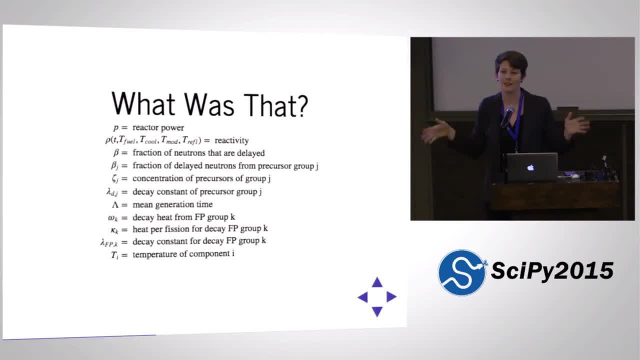 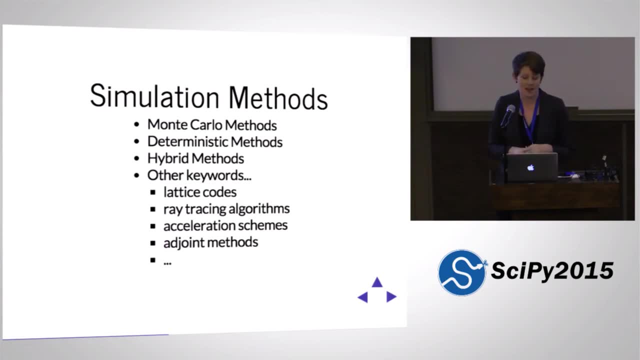 These all contribute to that equation and it's a big matrix like a set of PDEs, So you can do a whole bunch of different things to solve this set of PDEs. There's a lot of Monte Carlo that solves the static equation. 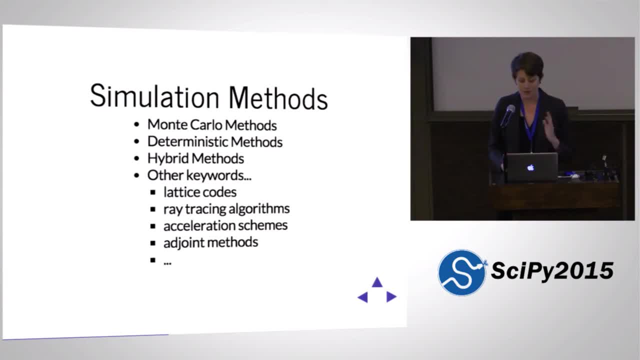 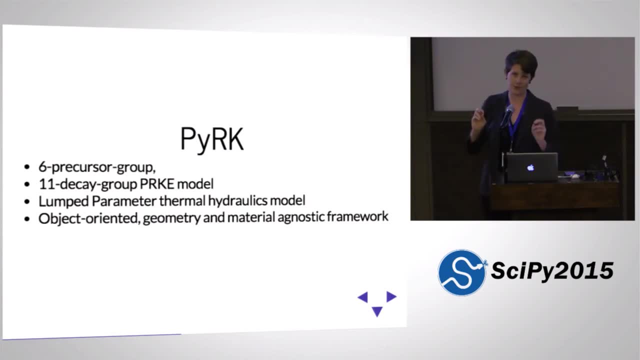 You can even use Monte Carlo and loop it to solve a dynamic version of the equation, And the possibilities are infinite. What we're going to use is a six precursor group, So the delayed neutrons come off of a certain set of isotopes. 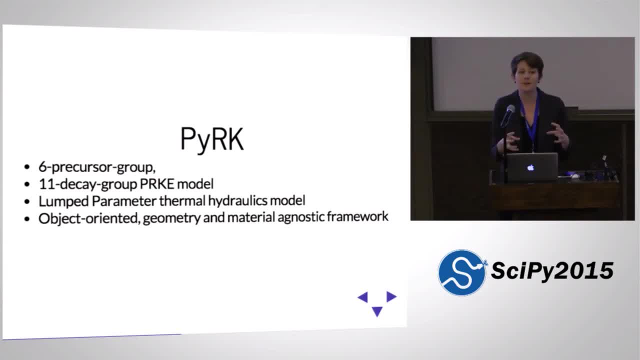 not all of them, just the ones that are unstable, And we're going to lump those into six different groups, which is a standard way of doing it, And so we're going to model all the delayed neutrons as if they're coming from six groups of isotopes. 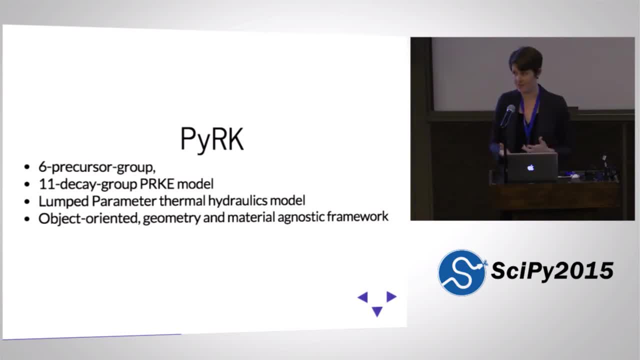 And 11 decay groups. so decay heat from fission also comes from all the isotopes, but you can lump them by their decay properties into 11 distinct groups, And so we're going to do that And we're going to model the thermal hydraulics. 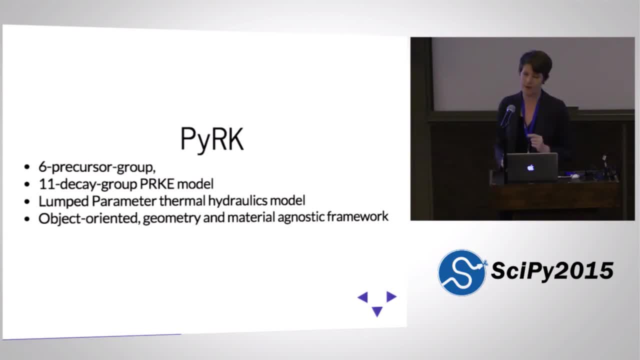 of how the temperatures respond to the power with a lumped parameter model which is super simple, sort of 1D approximation similar to a resistive circuit in electrical engineering, And we're going to put it all into Python and use Python's object-orientedness. 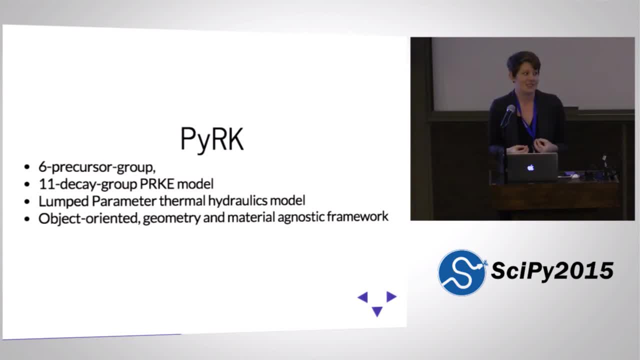 to make it easy to set up a simulation. So you can say: I want an object to represent the fuel and an object to represent the coolant. And those objects have attributes like their material isotopics and their cross-sections and their response to reactivity. 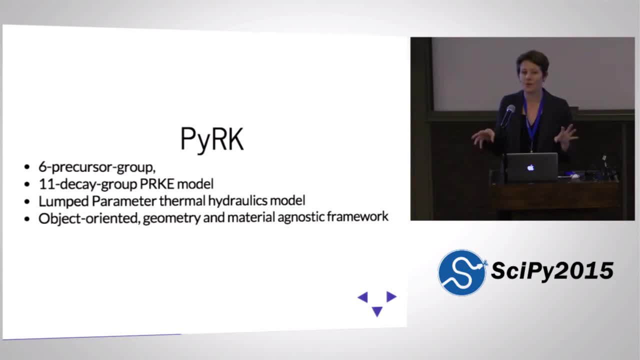 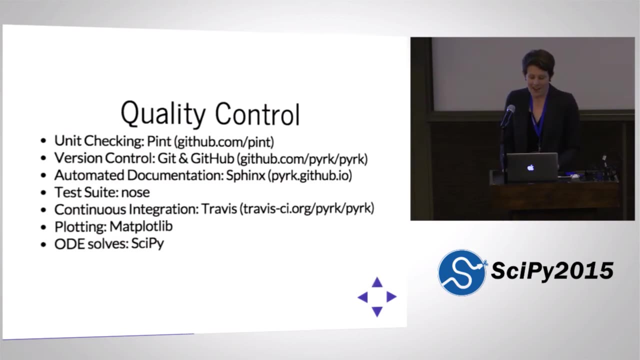 OK, And so all of that makes the whole thing a very geometry-agnostic framework and a material-agnostic framework, because you can load a material class to describe those components that you invent and add to PERC, So to make PERC work. 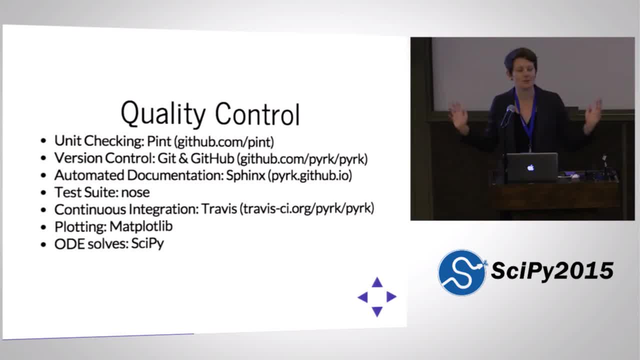 I tried to be as reproducible as possible and I used a whole bunch of tools from the SciPy stack, including one called Pint, which I discovered for this particular project and loved. So if you guys haven't tried it, it's called Pint. 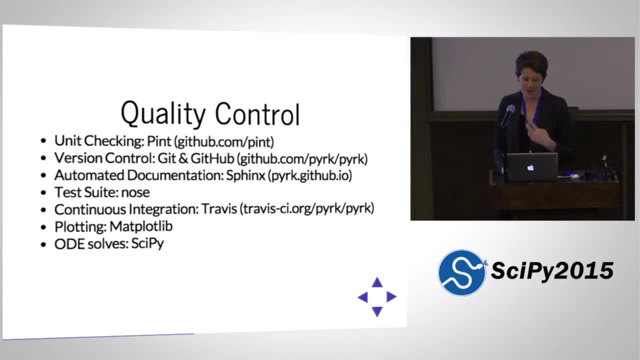 and it is a unit-checking software And of course I version control it with Git and GitHub. I document it with Sphinx, I test it with Nose, I have continuous integration in Travis plot with Matplotlib and I use SciPy to do most of my ODE solves. 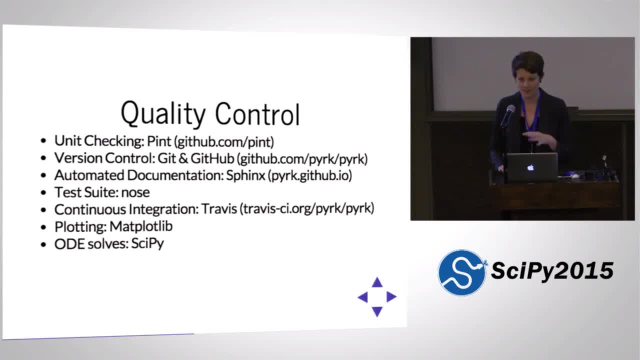 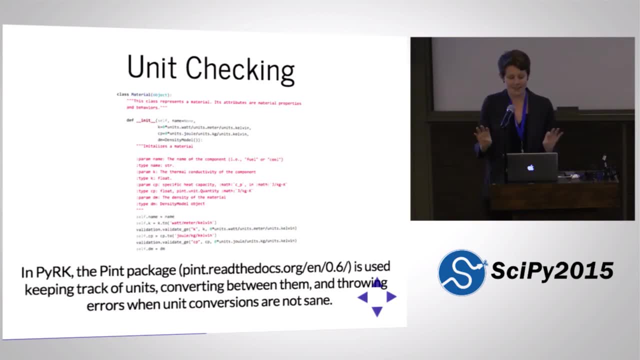 though the next version will include some like Katie Hough-specific ODE solves OK. So how does the unit-checking work? This is really small, but what's really cool is that Pint you associate units with each value. 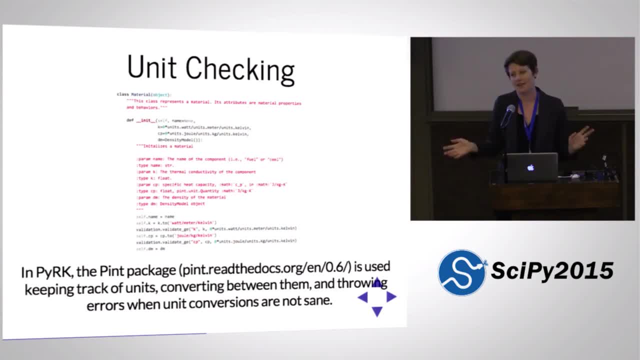 and they become quantities. And if you ever try to multiply two quantities to equal final quantity with incompatible units, Pint will complain and you don't have to set up your own whole suite of unit-checking in your code, which, as a physicist, is incredibly valuable. 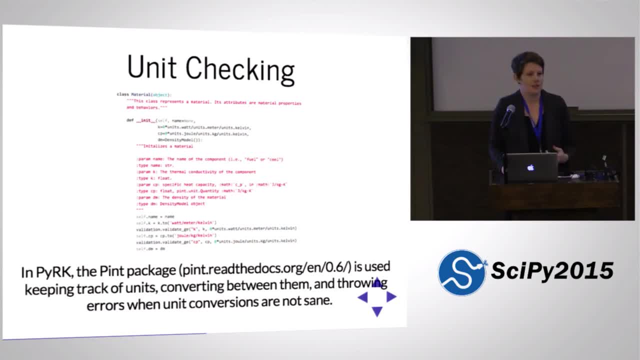 And in particular, as a physicist who's also an engineer. I encounter a lot of very complicated units that collide, So engineers and physicists don't always agree on what units to use, and it's really nice to be able to speak in both languages. 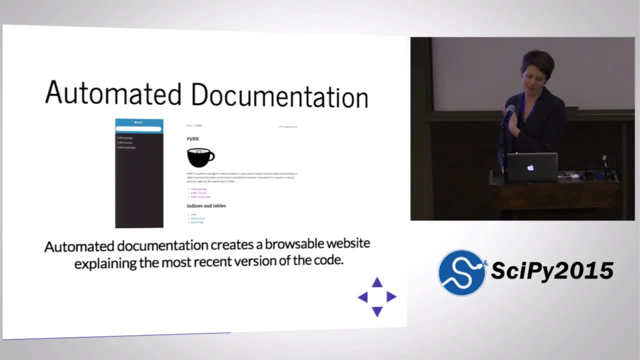 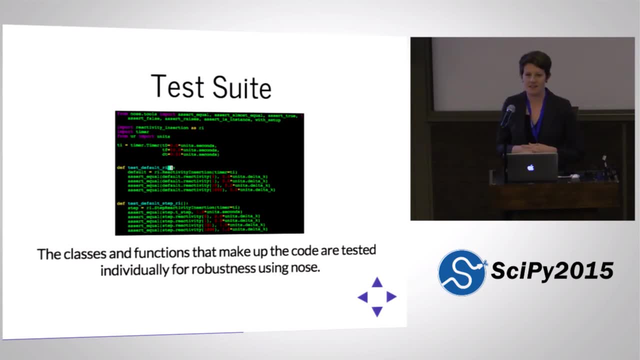 So version control with Git, it's all on GitHub, It's automatically documented. so we have a little website. We have a test suite. so, as I was saying, I use Nose and so I try to get some good coverage on my tests. 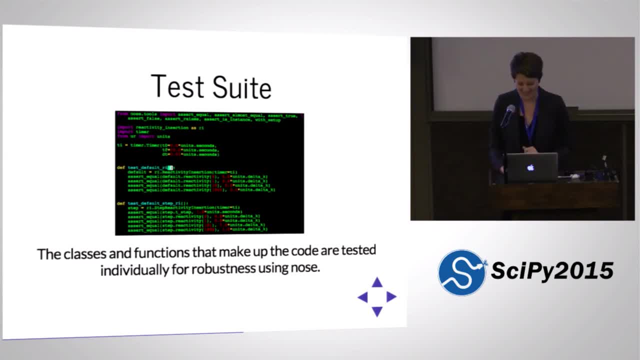 but I'm the only developer right now, so I don't have as much test coverage as I would like, so it's in my next version. We're currently in version 0.1, so this is a super, super alpha version of this code. 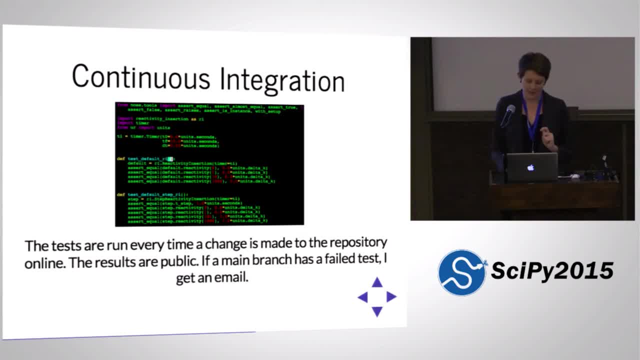 And all of that is continuously integrated on Travis. Oh, this is the wrong picture, but you guys know what Travis looks like. Travis is a continuous integration server, Right, And so all of this. how does it work? So let's talk about the stuff. 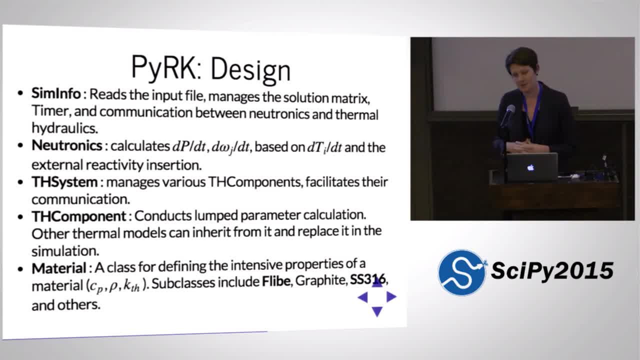 that you guys are interested in. So the way that this is designed, it has a singleton simulation information object that collects the input from a single input file where the engineer can set up their simulation name. those objects create a fuel object, give it attributes. 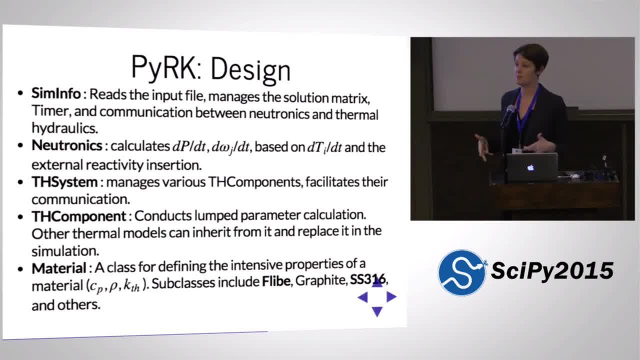 like it's cross-section behavior. and then you know you can use that to create a single input file where the engineer can set up their simulation name those objects: create a fuel object, give it attributes- like it's cross-section behavior. 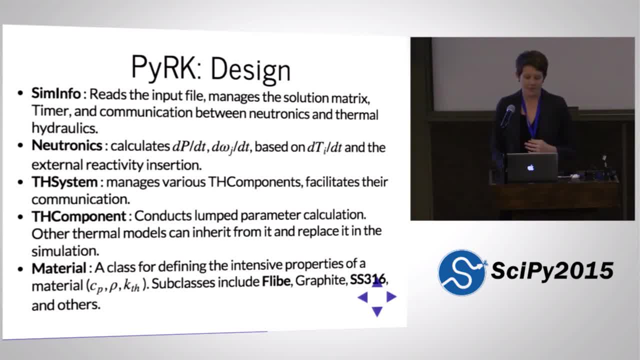 and then you know, give it attributes like it's cross-section behavior, and that simulation object then creates a neutronics system and a thermohydraulics system and runs the communication between those things in order to do the ODE solve. 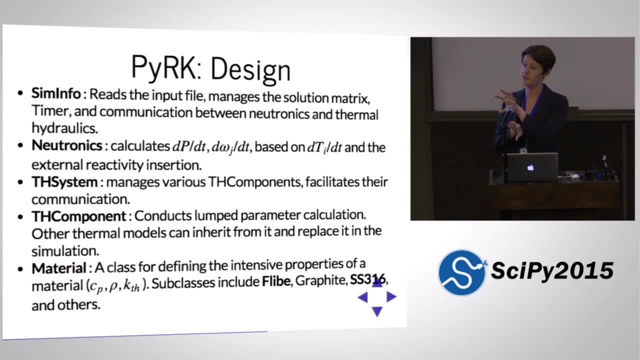 of that big matrix which is a combination of neutronics and thermohydraulics. The neutronics system mostly calculates the change in temperature, the change in decay heat and the change in reactivities based on the temperature and that any external reactivity insertion. 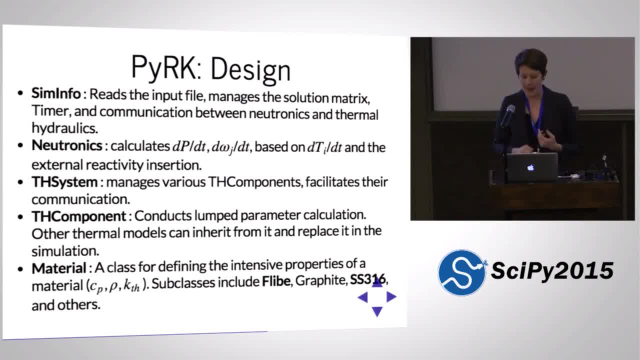 that the simulator likes to like wants to do. So. you know, it's a combination of neutronics and thermohydraulics based on the temperature, and that any external reactivity insertion that the simulator wants to model, And by the simulator 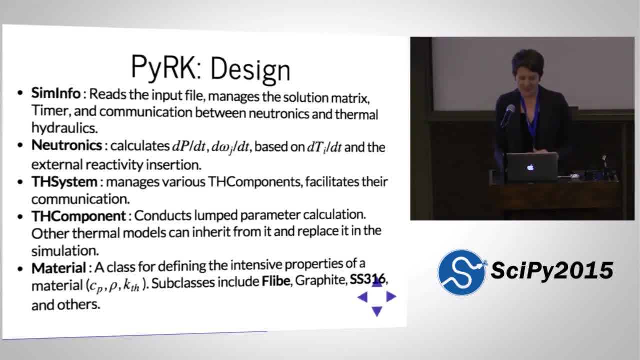 I mean the user. The TH system manages various thermohydraulic components, so those things that respond with the temperature and then feedback to the reactivity, and the components themselves are the objects that the simulation runner, the user, has defined. Each of those, 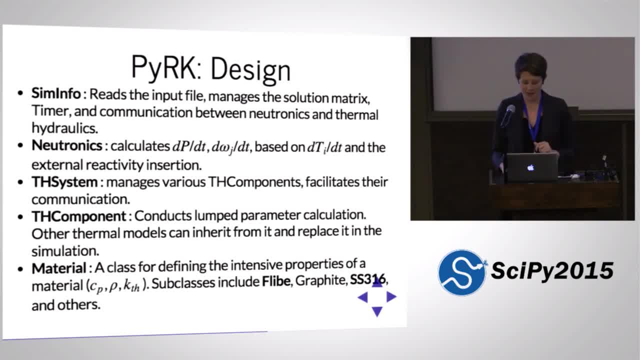 TH components, like I said, has a material, and that's a very important part of this. These classes right now include a number of different components that are used to include various materials that I'm interested in, including flibe, which is a type. 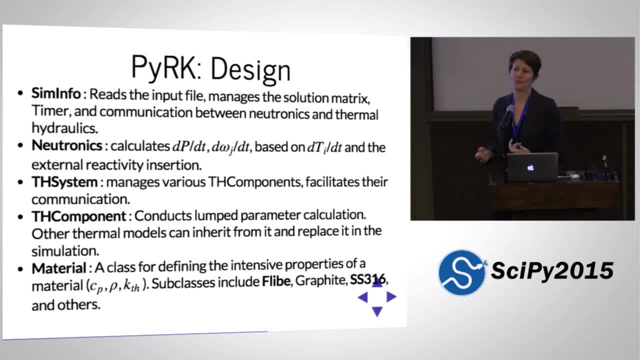 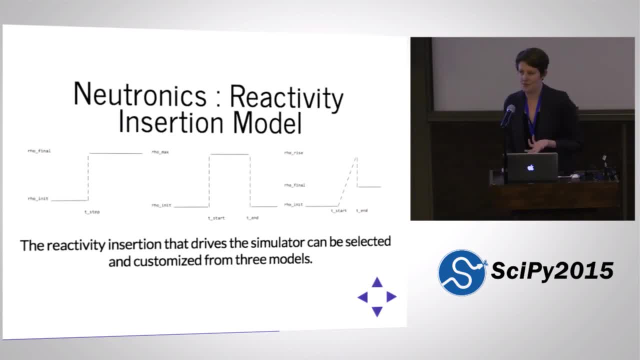 of salt and graphite, which is graphite, and stainless steel 316,, which is a really common nuclear grade steel, and a lot of others. But just keep in mind that you can add any material class that you want, because it's open source. 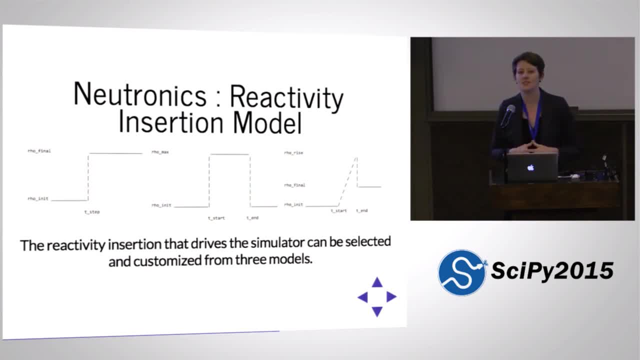 and it's a really simple API for the material class Okay Neutronics itself. the simulations right now in version 0.1 can only be driven by reactivity insertions. There's a lot of types of accidents and transients that can happen. 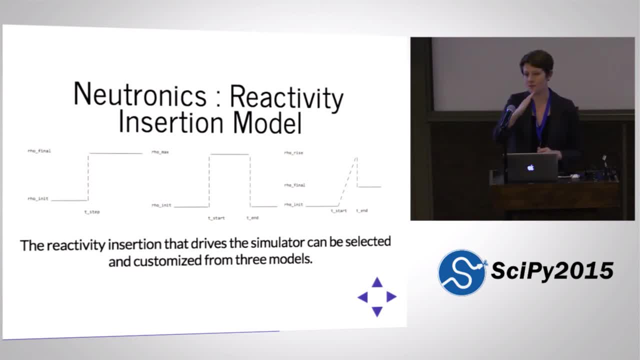 in a nuclear reactor. These include start up and shut down, where the reactivity changes from zero to critical or critical to zero, And they also include accidents where the coolant stops moving or you drop a control rod, And right now PERC can only model. 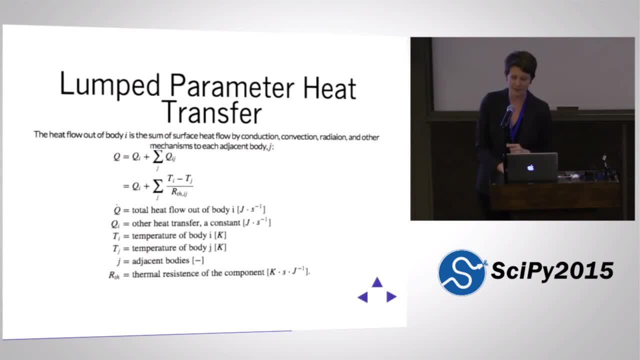 the dropping, a control rod type where you insert some external reactivity, But in the future it will include more: The lumped parameter heat transfer model. I'm not gonna go into the math. it's a circuit and it assumes that all the components 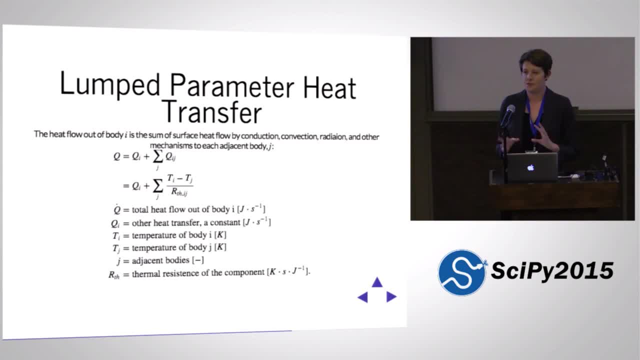 are lumps. It has a constraint: You only wanna use it for certain sizes of lump. It has a Biot number constraint, But you can split any lumped object into many small lumps and it'll become valid again. So you wanna use it. 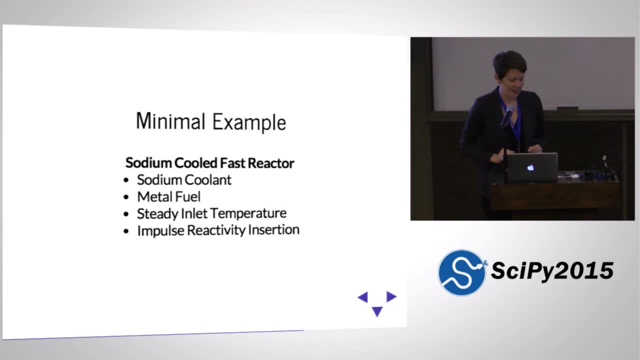 in a valid way, or else you'll get the wrong answer. Okay, Now that I have only a couple of minutes, I will give you just the minimal example of what PERC actually does. So, given all that background and given the fact that it's a transient, 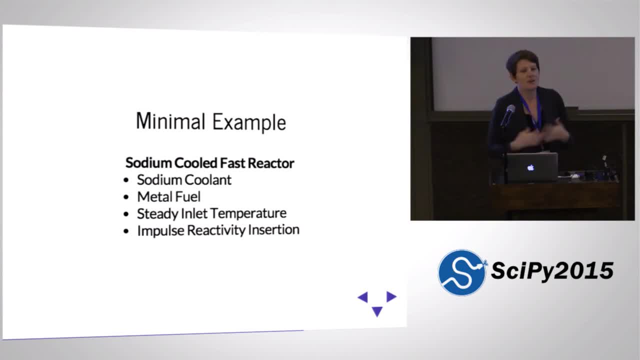 and it can do these reactivity insertion accidents. one of the kinds of things that, in fact, the kind of thing that you wanna do as a nuclear reactor engineer, in particular a designer of nuclear reactors, is prototype various reactor designs and see how they respond. 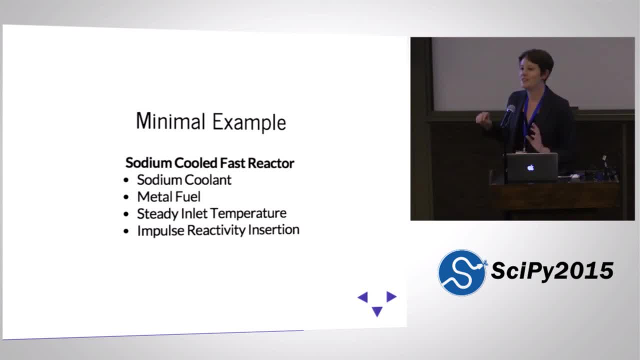 to accident transients. And so let's take a typical advanced reactor design that's supposed to respond beautifully to an accident. So a sodium cooled fast reactor is a super cool, super cool type of reactor that, because of its inherent physics, in an extreme reaction situation. 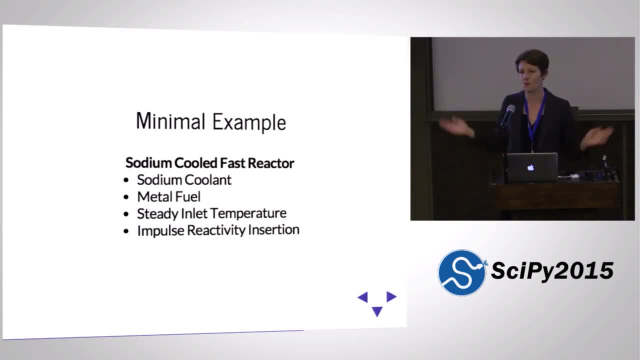 where, like you introduce a whole bunch of extra reactivity, it shuts itself back down to a normal power, which is actually really wonderful and beautiful And that's entirely based on the physics. So the pieces of this is: I've got a sodium coolant. 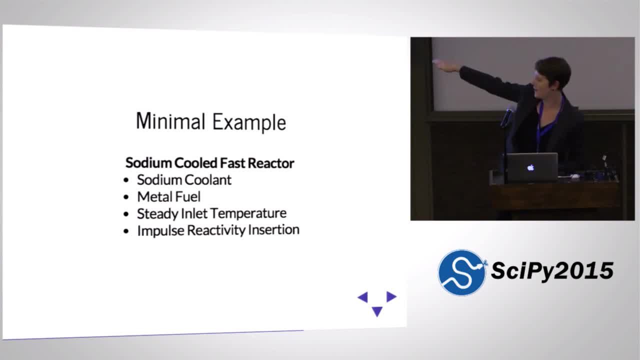 a metal fuel and I hold the inlet temperature steady, And this is just a really toy example. And then I drop, I pull out a control rod, so I increase the reactivity. and then I drop a control rod and I increase the reactivity. 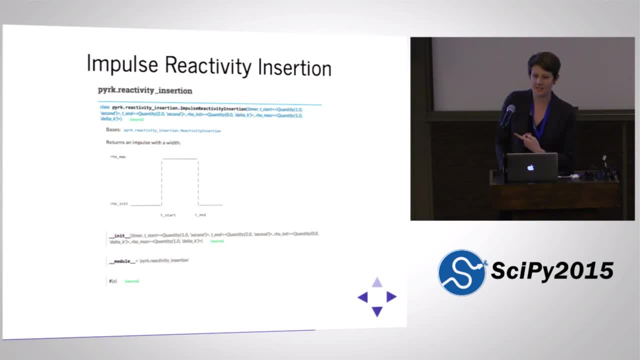 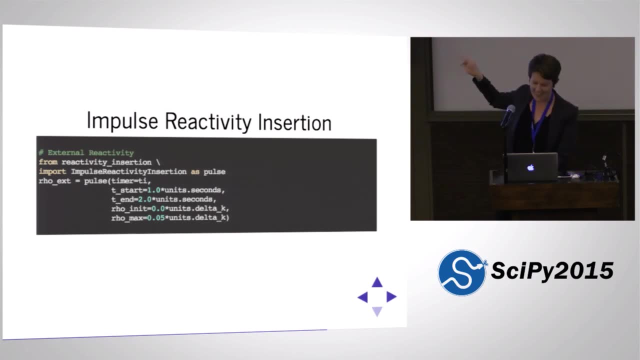 And then I drop it back in a second later And that dropping looks like this: So here's the docks for the reactivity insertion. I use this information. I put a little function- excuse me- into the. I put a little function into the input file. 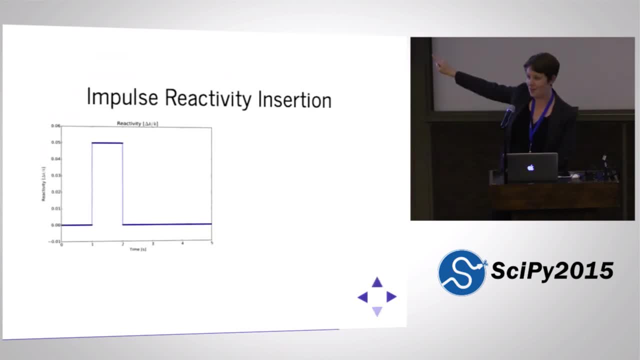 to represent that. And then I get out as the response in this simulation a reactivity insertion And it looks just like I was expecting And the response from the power incorporates the temperature response that we were expecting and some of the reactivity response. 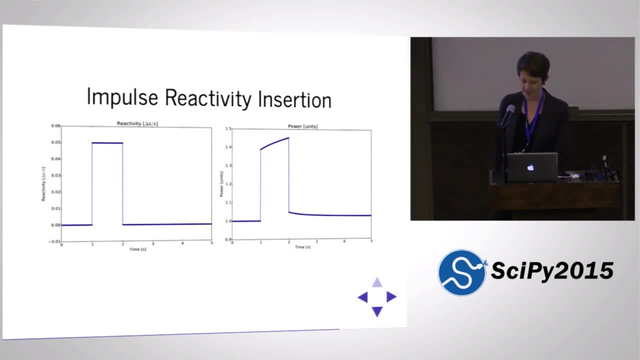 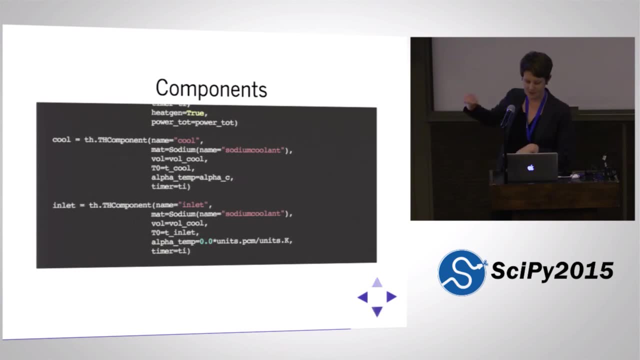 Anyway, I then drop back in the control rod and you can see the transient ends. I add the components in this way. This is what the input file looks like when I add a fuel and a coolant and an inlet. I won't go into it.